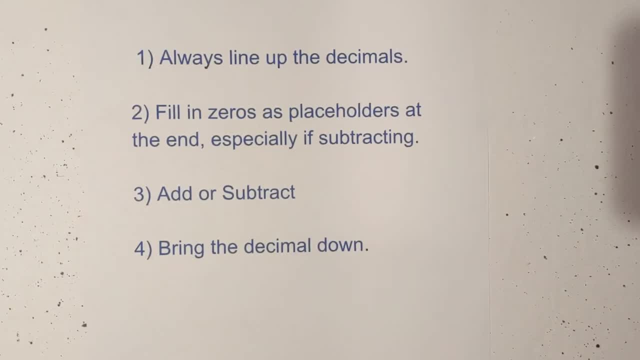 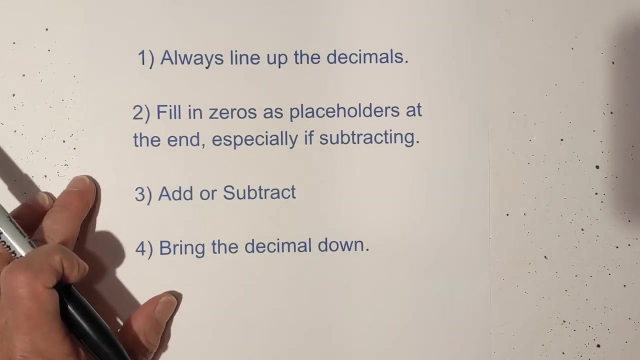 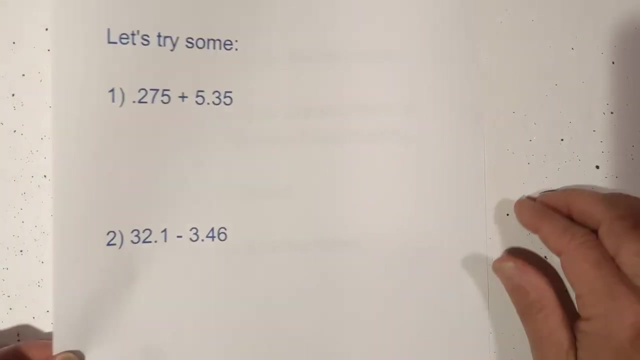 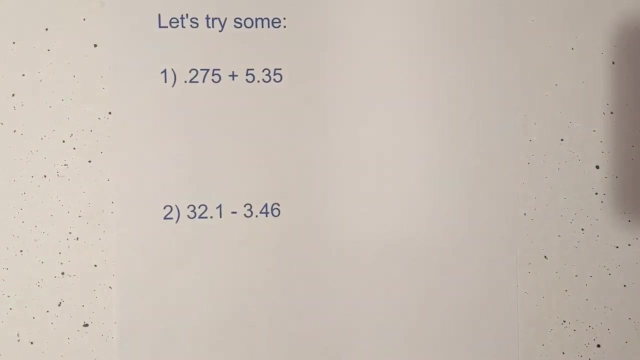 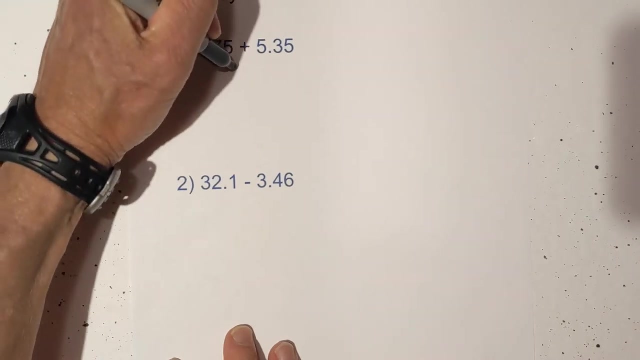 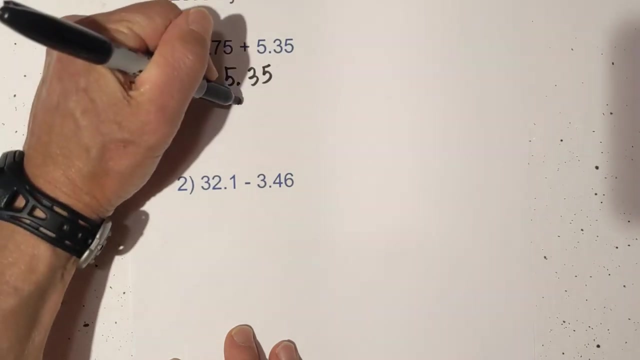 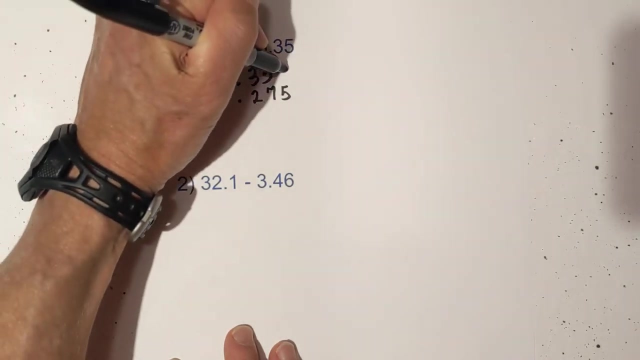 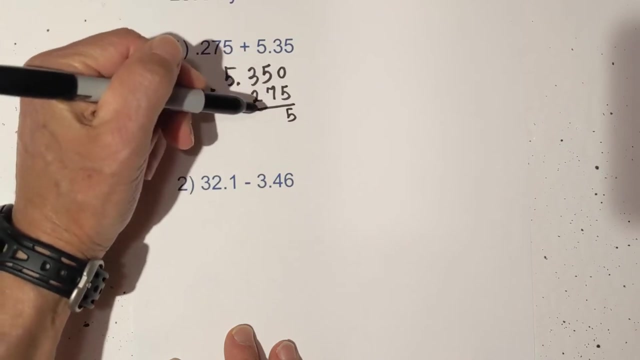 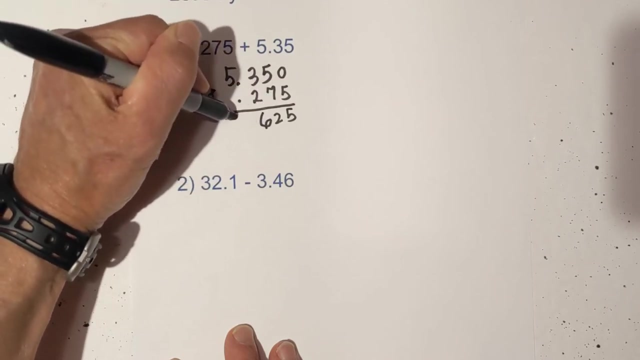 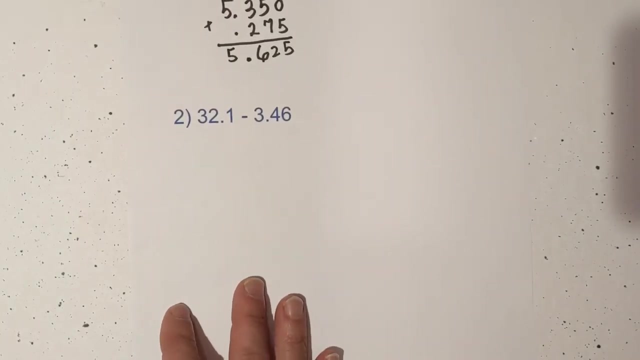 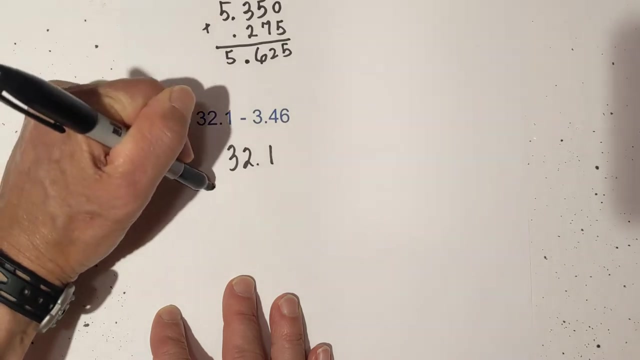 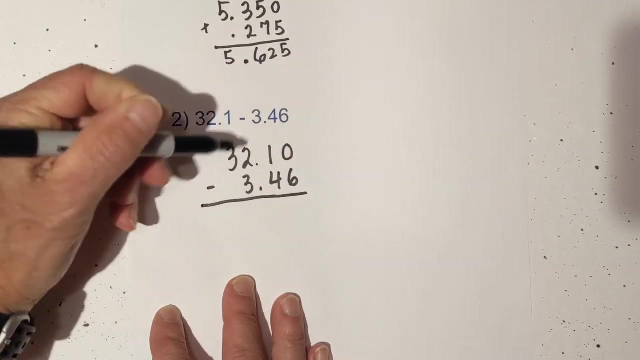 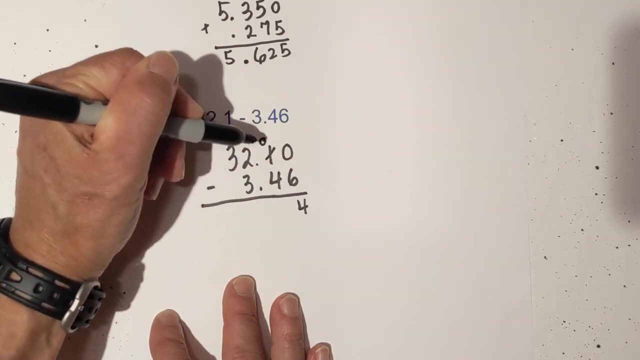 Welcome to MooMooMath and Science. In this video let's learn how to add and subtract decimals and here's what we're gonna do we're always gonna line up the decimals we're gonna fill in zeros as placeholders at the end especially in subtracting and then we're gonna add or subtract and we're gonna bring the decimal down so let's get started here's problem number one okay so we have 0.275 let me get this out from underneath okay we have 0.275 plus 5.35 so let's go ahead and write this and I'm gonna write the 5.35 up top because I just think that will make it easier then the decimal is right here we're gonna line up the decimals two seven five okay I'm gonna fill in zero as a placeholder then all we do is add that's five that looks like 12 carry the 1 3 4 5 that's 6 there's 5 and then we're gonna bring down the decimal so it's 5.625 now let's try some subtraction so what we have is we have 32.1 minus 3.5 4 6 let's put in a 0 okay now what all we do is subtract this will be a 4 I'm gonna borrow 10 from here so this will be a 0 this will be a 6 I had to borrow 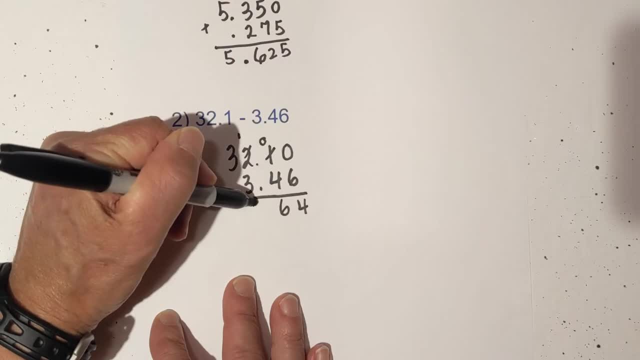 10 from here so that would be a 1 so that becomes an 8 and I had to borrow 1 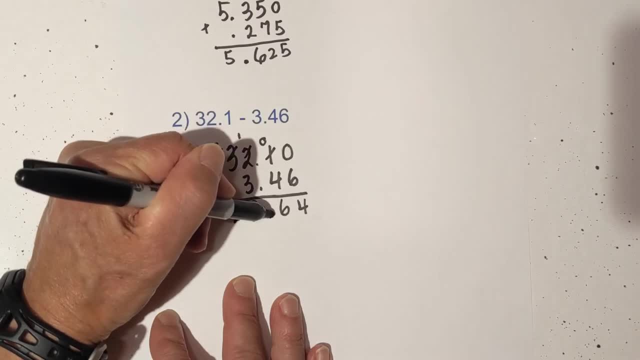 from there so that becomes a 2 bring down the decimal there's 228.64 so let's 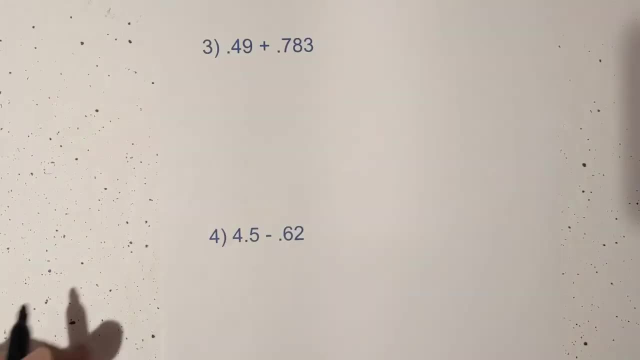 go ahead and move on to the next problem number two we're gonna write this down we're gonna move on to a couple more Okay 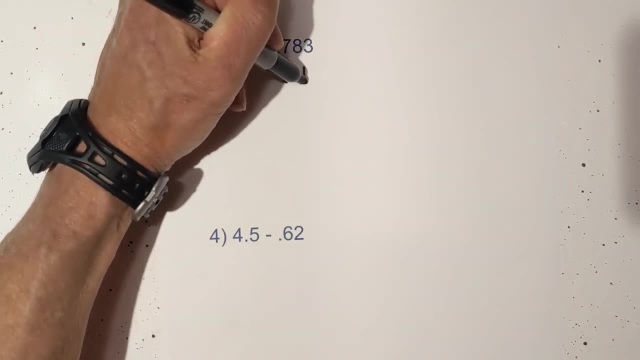 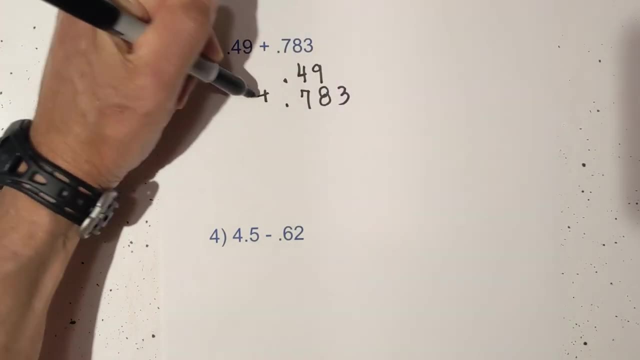 Here we go again I'm gonna write them and remember we line up the decimals okay then this is addition I'm going to fill in the placeholders. Okay so,